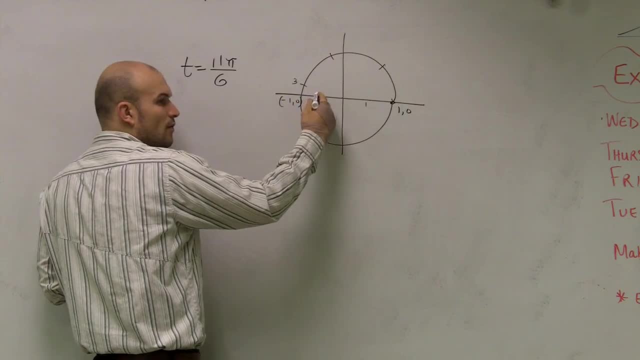 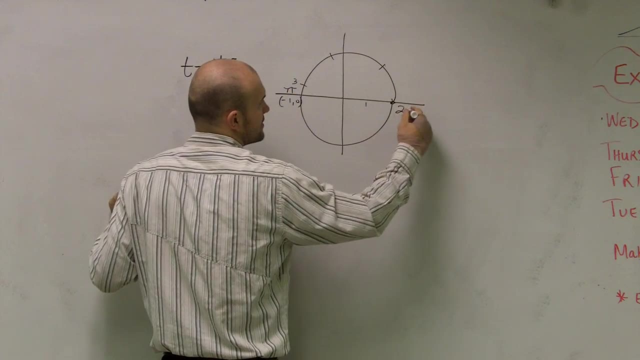 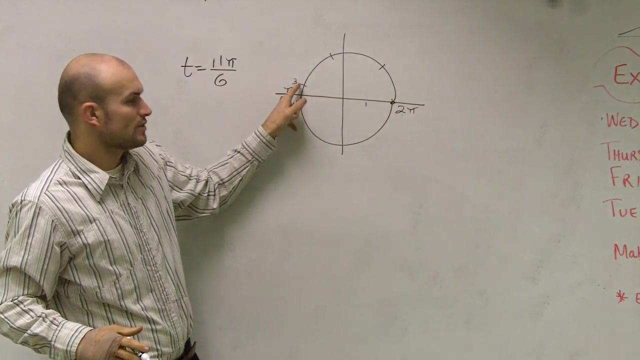 So at this point we said: this is what we call 3.14159, or what we would call pi Radians. And then, if I was to go around again, I'm just going to kind of raise this here- we're at 2 pi, right, That's 2 pi radians. This would be 1 radian, 2 radians, 3 radians and then all the way around, halfway around would be 3.14 radians, which we just label as pi. 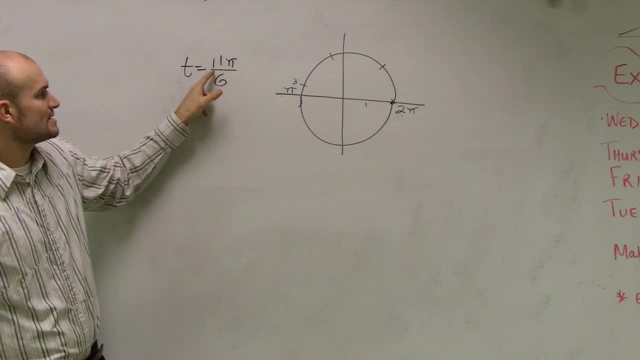 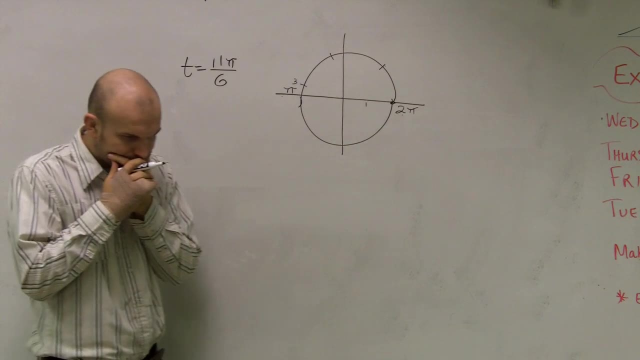 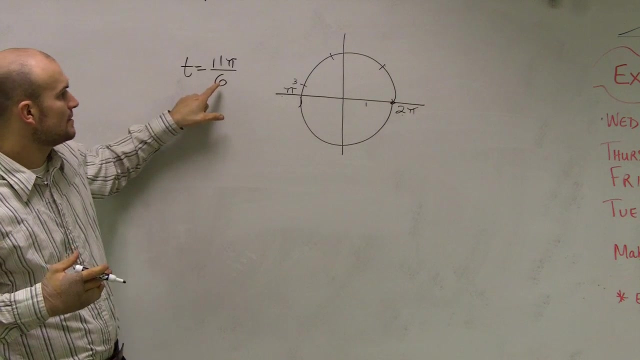 So this one says they wanted to determine this in 11 pi over 6.. So, um, when doing 11 pi over 6, what I like to do for these types of problems is: I want to cut. remember, guys, if this is 11 pi over 6, I could say that 6 pi over 6 is the same thing as pi, right? 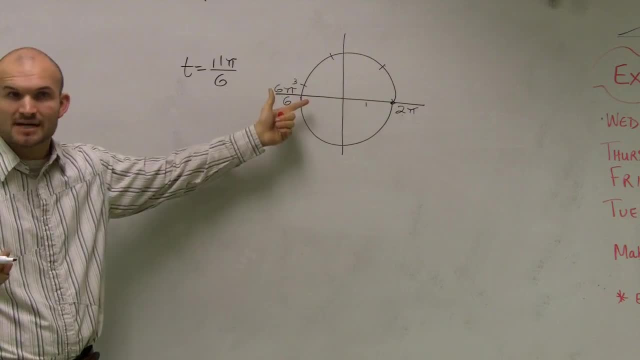 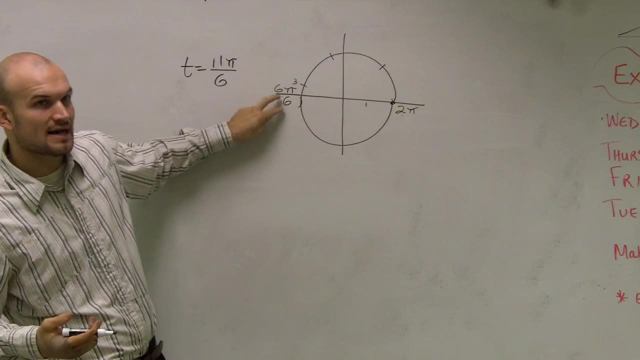 Because 6 divided by 6 is still is 1, 1 times pi is pi. So when I'm solving one of these problems, I like to always take my ratio, what my denominator is, and rewrite pi with that denominator. 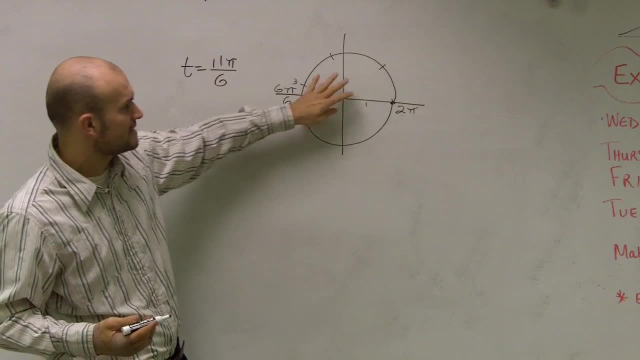 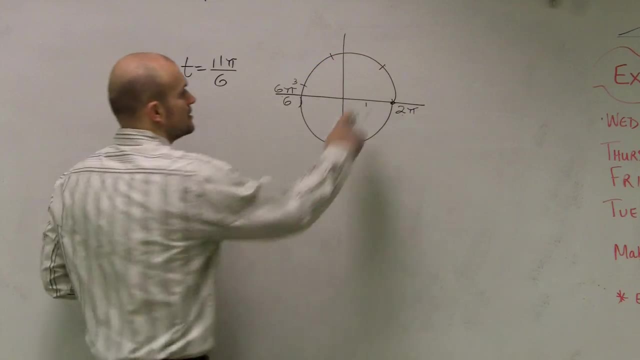 So if this is 6 over 6,, what I'm going to want to do is now separate. I'm going to want to like cut out my- uh, my unit circle into 6.. So I'm just going to kind of forget about the radians here for a second and let's break this up into 6.. 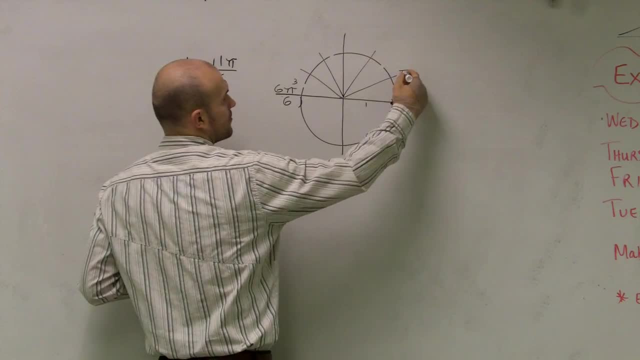 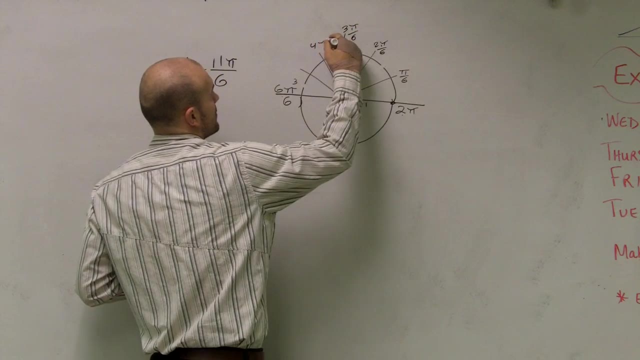 And I know I'm not going to be perfect. so therefore, this would be 1 pi over 6,, 2 pi over 6.. 3 pi over 6,, 4 pi over 6,, 5 pi over 6,, and that's 6 pi over 6.. 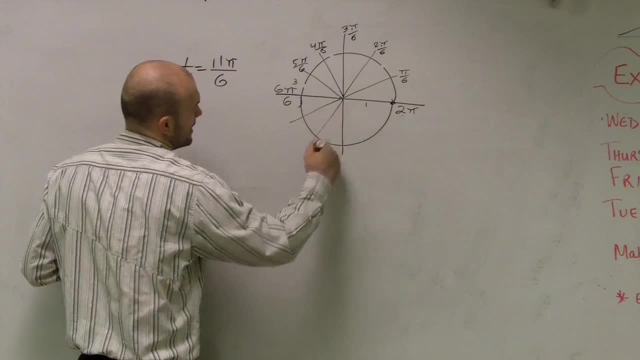 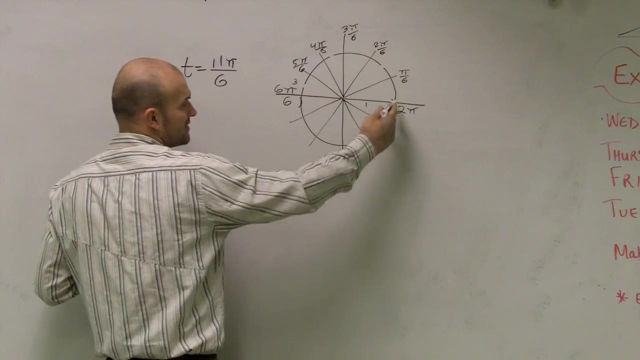 Does everybody see that? And it's obviously you can go 7,, 8,, 9,, 10,, I'm sorry, I'm sorry 7,, 8,, 9,, 10,, 11,, 12.. 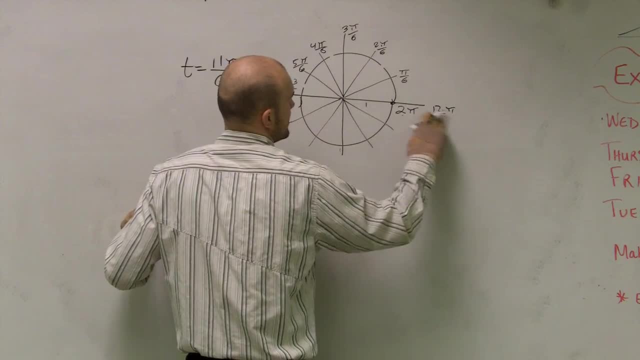 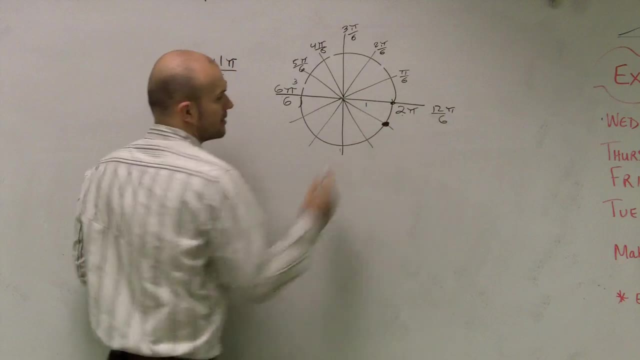 Well, is 12 pi over 6 the same as 2 pi? Yes, it is right. So they're asking: where is 11 pi over 6?? Well, that's going to be this point, right here. Okay. 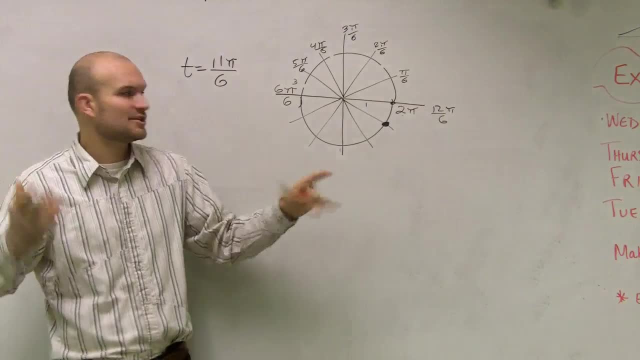 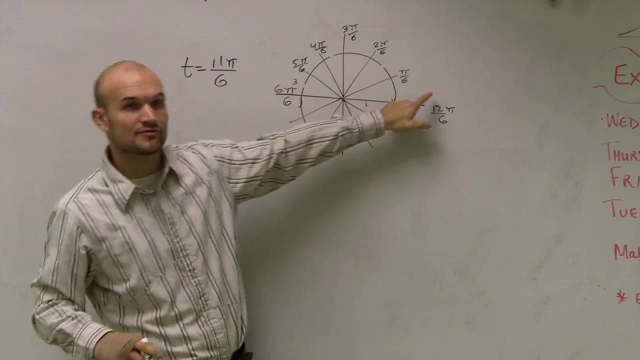 That's step number one. You guys have to know how to determine where they're at. The easiest way to do it is to section off your unit circle into what your denominator is Done And also make sure it's the positive direction. That's why I went this way. 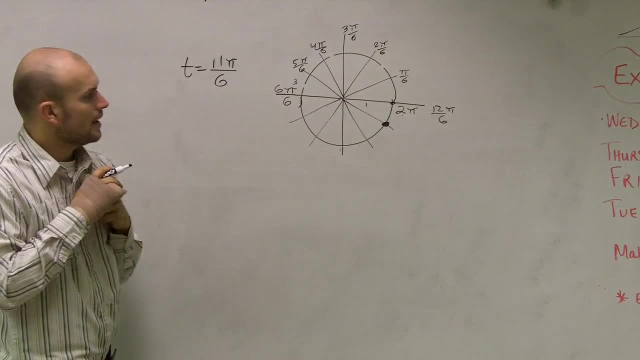 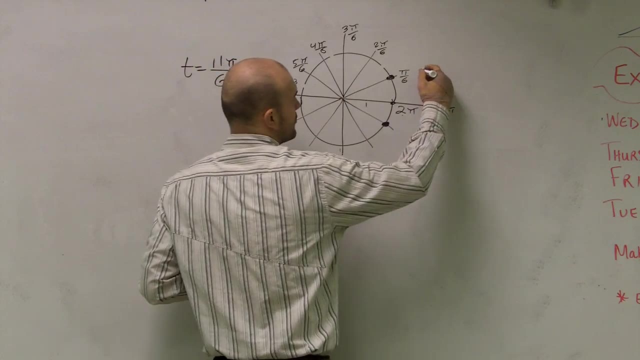 If it was negative, we would have gone in that way. The next thing is we need to determine what is the coordinate point. Well, by using our unit circle, all right, we know that this point is square root of 3 over 2 comma 1 half. 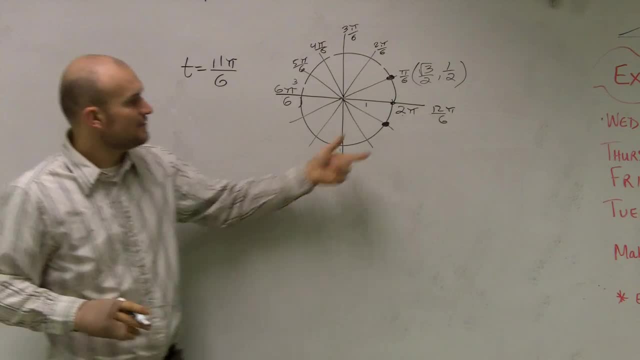 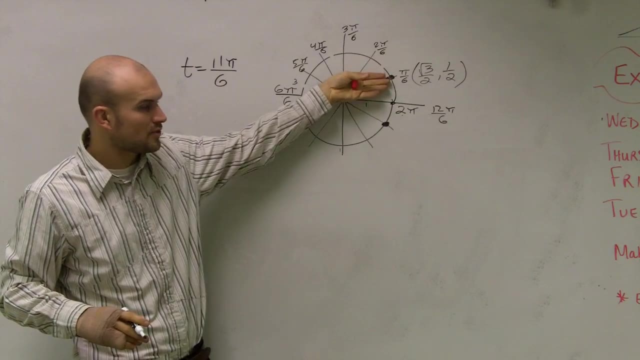 Okay, All right. So then, if you guys kind of notice, these two points are kind of a reflection of each other, aren't they Right? You can kind of take this point, reflect it over your x-axis and you get to this point. 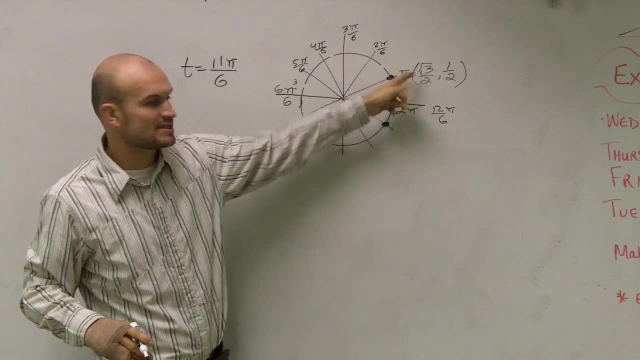 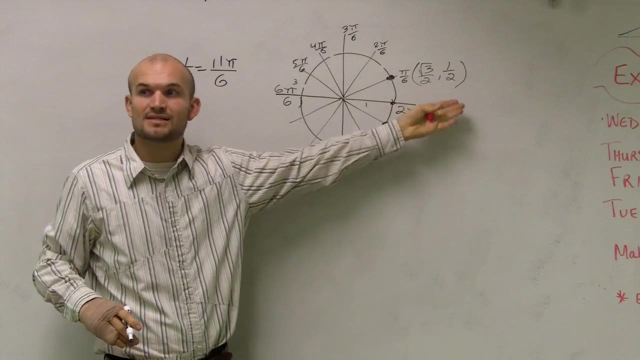 Does everybody see that? So what does the only thing change? The x value is still not going to change. It looks like the x value is the exact same point, But the y value is now going to change and it's going to become, instead of a positive, it should become a negative. 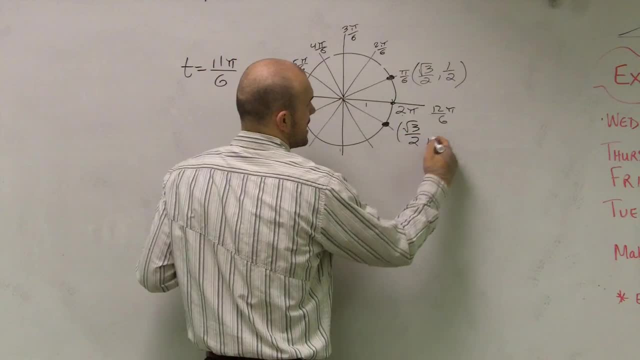 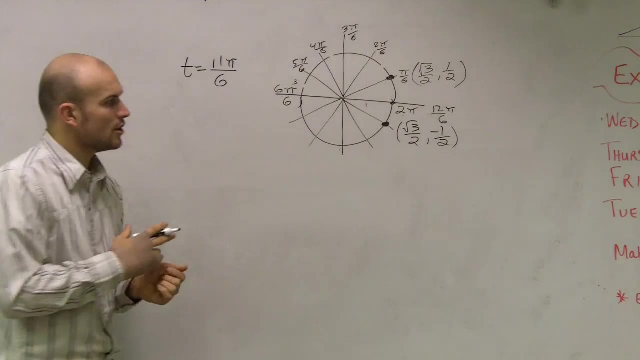 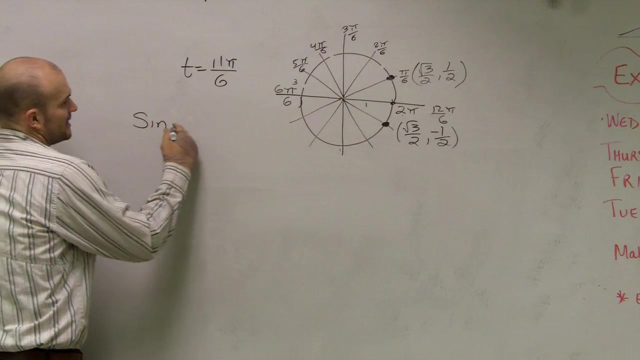 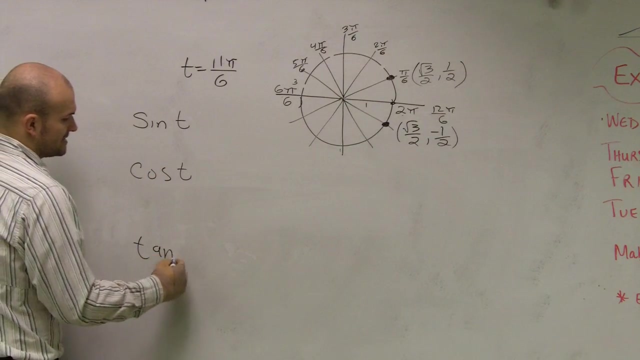 So this point is square root of 3 over 2 comma, negative 1 half. Does everybody see that? Okay, So that's step number two is finding your coordinate point. Now the next thing we need to do is we need to evaluate sine of t, cosine of t and tan of t. 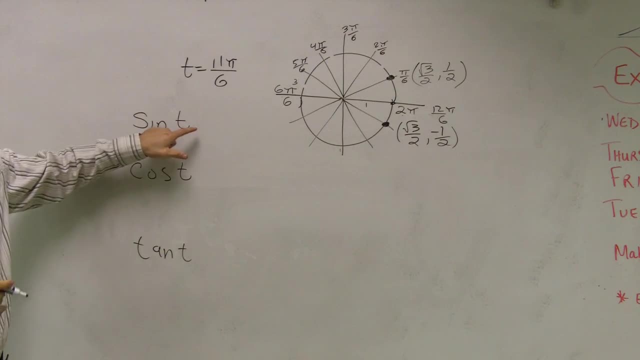 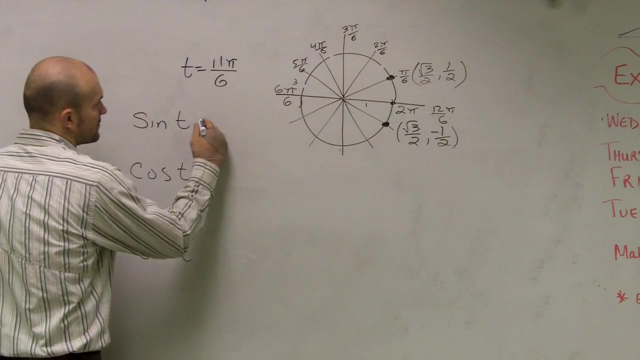 Well, a couple of things you guys need to remember. Sine of t is equal to y, the y coordinate of your point t. So my y coordinate of my point t is equal to y And my coordinate of my point here is negative 1 half. 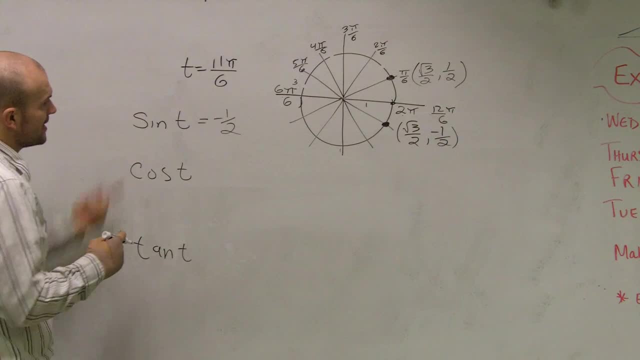 And cosine is going to be x And cosine And actually my t also. we can evaluate this. We can also say this is going to be 11 pi over 6, right, Because you know that sine of t equals y. 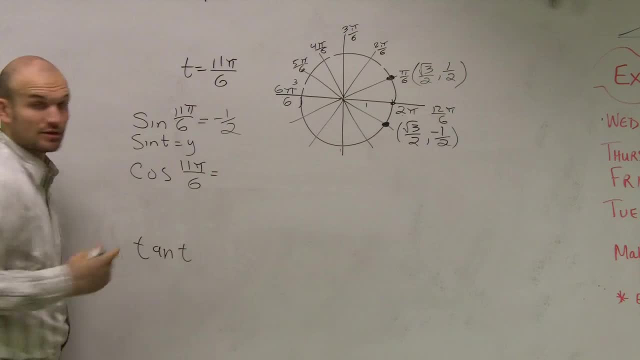 So cosine of 11 pi over 6 is equal to the x, which is root 3. Over 2.. Because cosine of t is equal to the x coordinate And tangent- this one's going to get fun here. Tangent is going to be your y over x, when x cannot equal 0. 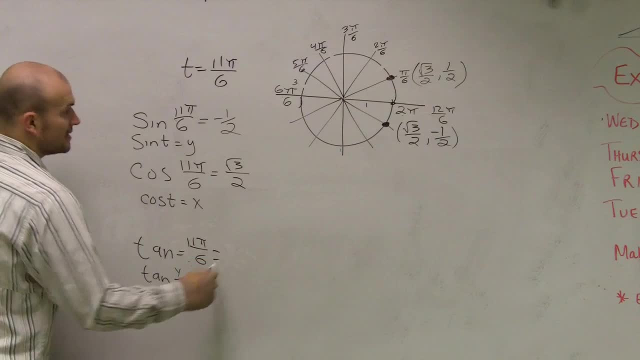 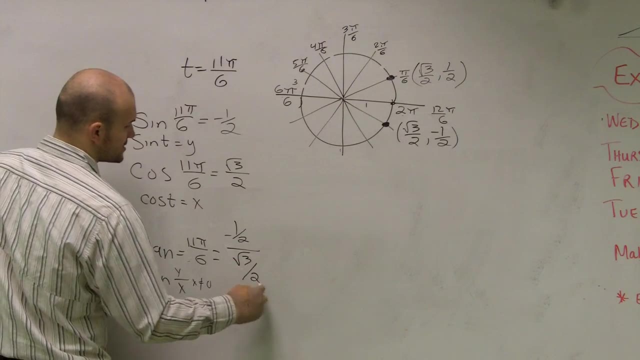 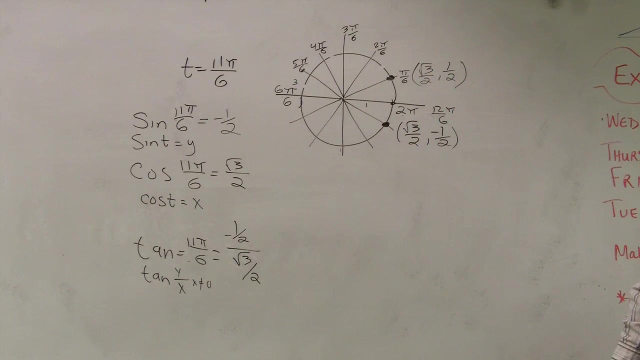 So tangent of 11 pi over 6 is equal to my y, which is a negative 1 half divided by root, 3 divided by 2.. Okay, Isn't the cosine supposed to be radical, 2 over 3? No, 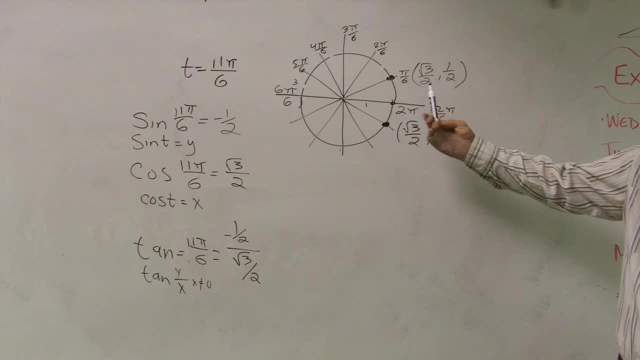 I think you might get confused with 4.. I think on the unit circle it's radical 3 over 2.. But for pi over 4, it's square root of 2 over 2.. Is that what you're looking at?